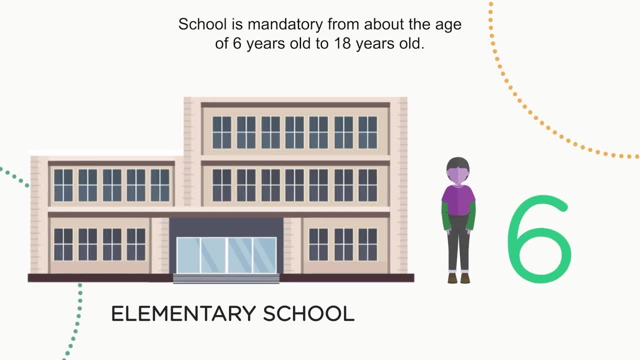 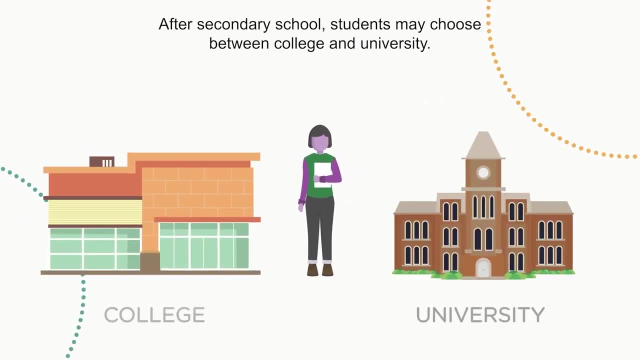 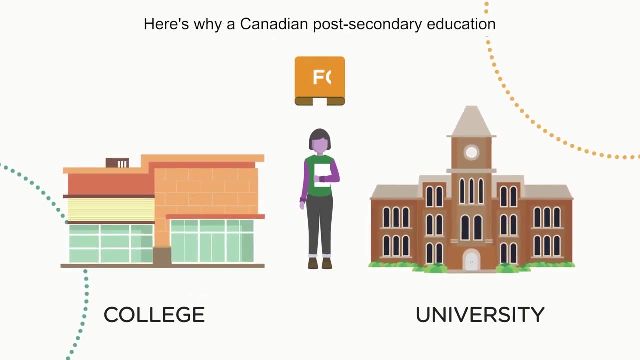 School is mandatory from about the age of 6 years old to 18 years old. After secondary school, students may choose between college and university. Both education systems help students prepare for their future. Here's why a Canadian post-secondary education may be a great choice for your future. 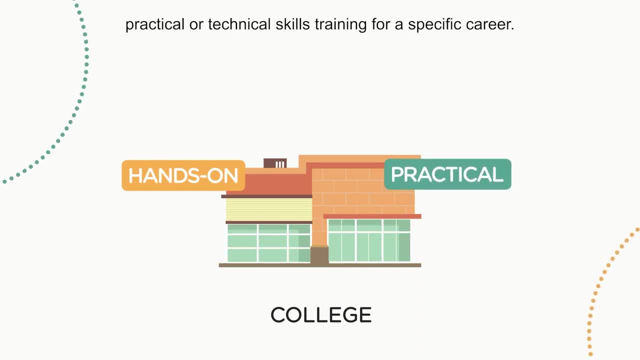 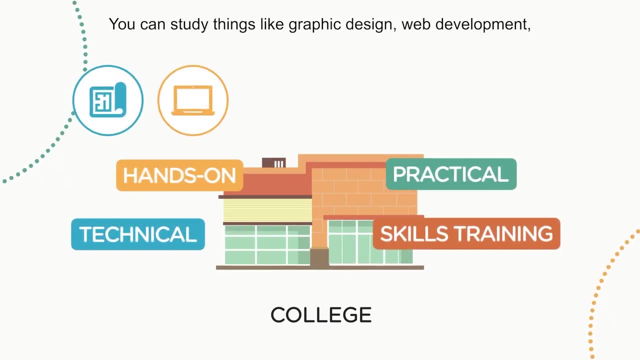 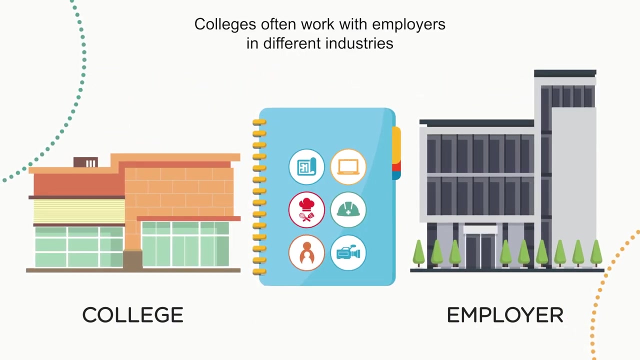 At college, students can get hands-on practical or technical skills training for a specific career. You can study things like graphic design, web development, culinary arts, occupational health and more. Colleges often work with employers in different industries to develop the latest curriculum. 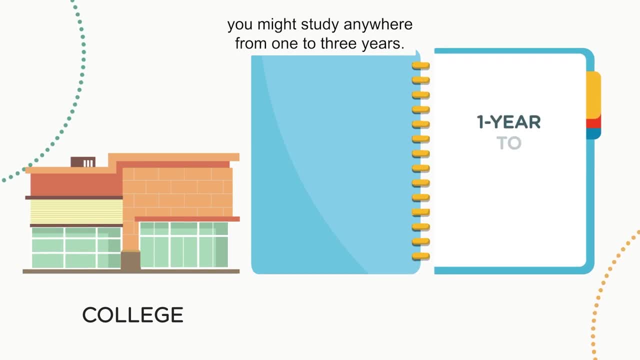 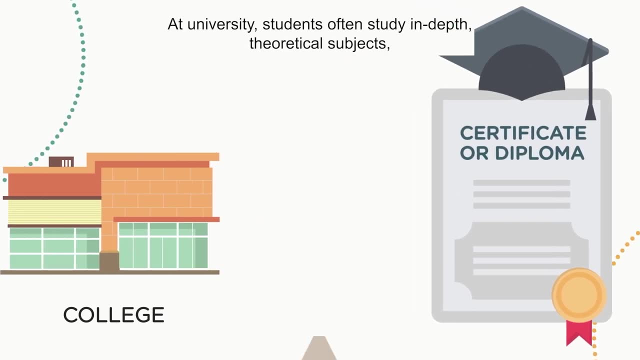 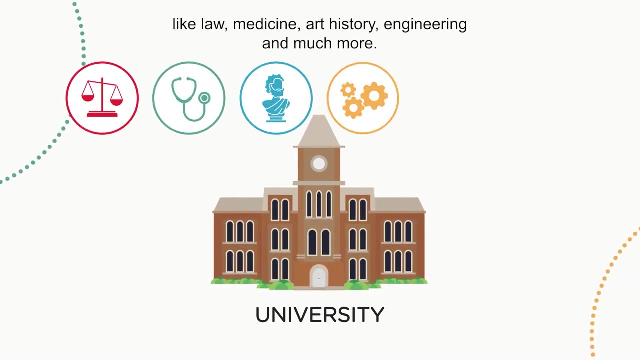 Depending on your college program, you might study anywhere from one to three years. When you graduate, you'll receive a certificate or diploma. At university, students often study in-depth theoretical subjects like law, medicine, art, history, engineering and much more. 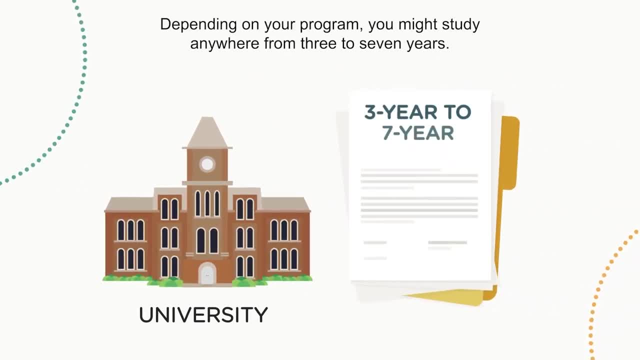 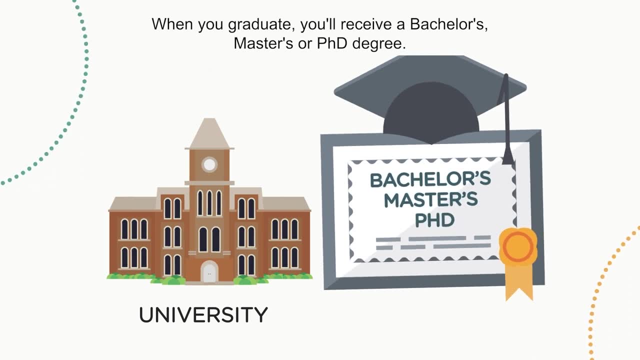 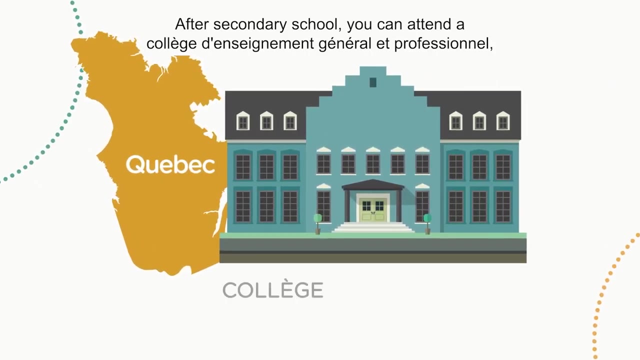 Depending on your program, you might study anywhere from three to four years. When you graduate, you'll receive a bachelor's, master's or PhD degree. In the province of Quebec, the education system is unique. After secondary school, you can attend a collège d'enseignement général et professionnel known as CEGEP. 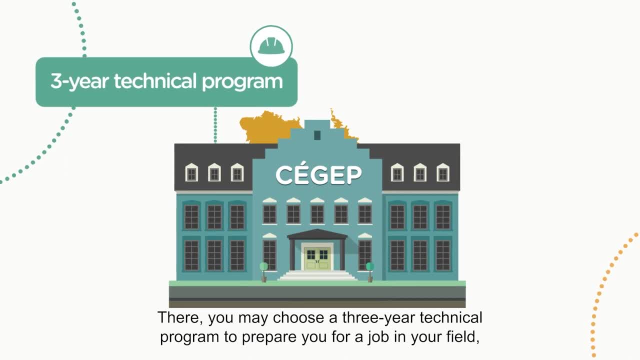 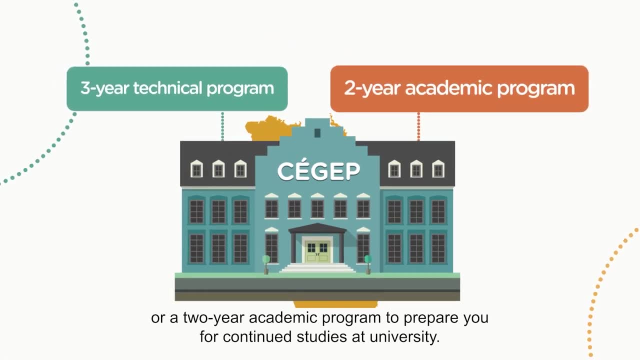 There, you may choose a three-year technical program to prepare you for a job in your field, or a two-year academic program to prepare you for continued studies at university. No matter in which province you study, choosing between college and university depends on your interests and goals. 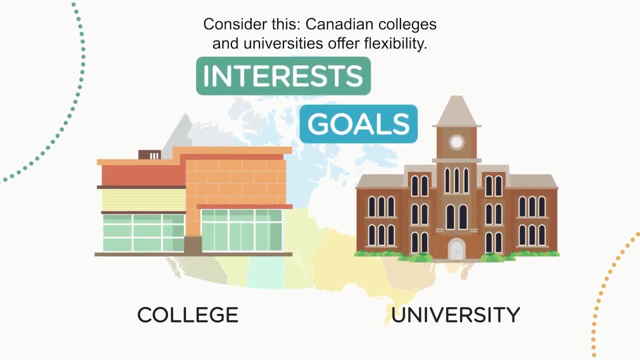 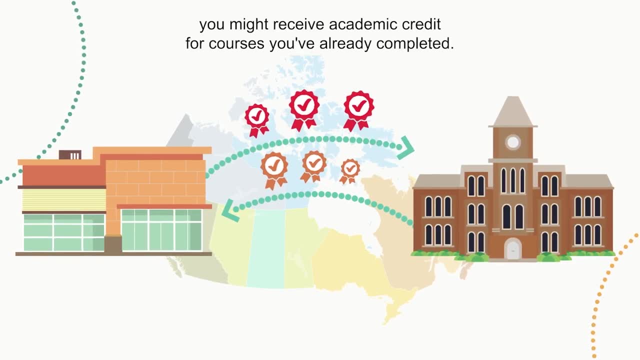 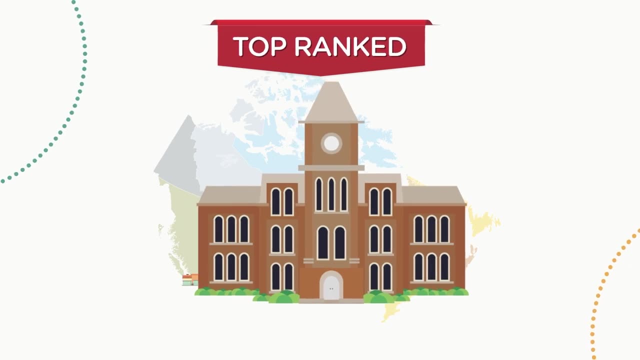 Consider this. Canadian colleges and universities offer flexibility: If you study at one school and wish to transfer to another, you might receive academic credit for courses you've already completed. Several of Canada's universities appear on well-known university rankings lists. Some Canadian college and university programs offer cooperative or work-internship programs. 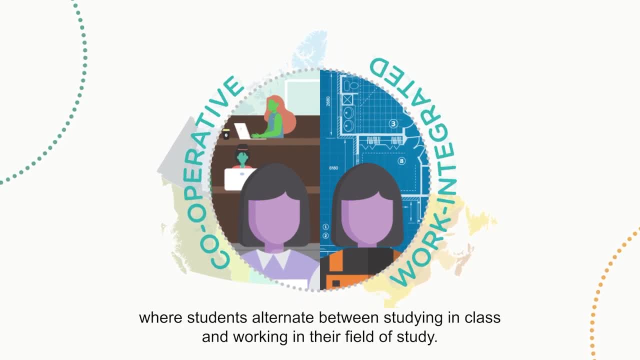 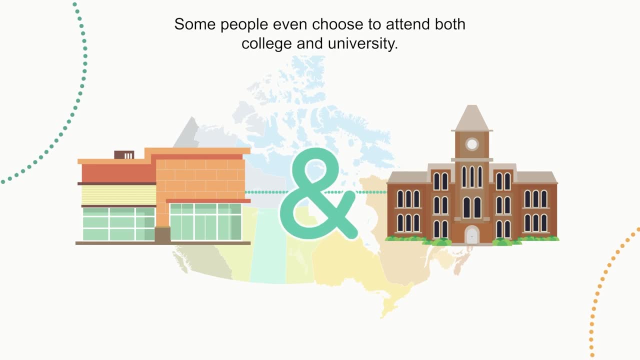 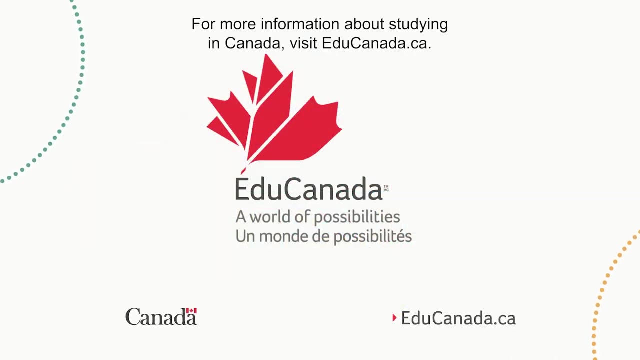 Some are integrated learning experiences, where students alternate between studying in class and working in their field of study. Some people even choose to attend both college and university. Whatever your choice, Canada is a great place to study. For more information about studying in Canada, visit educanadaca. 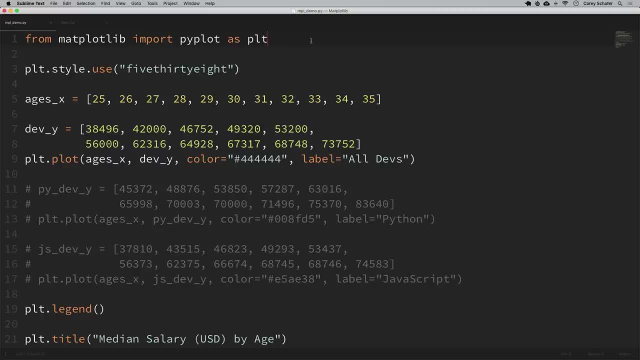 Hey there, how's it going? everybody, In this video we're going to continue learning about Matplotlib and seeing how to create some different types of charts. Specifically, we're going to be looking at bar charts. in this video, We're also going to see how to load in. 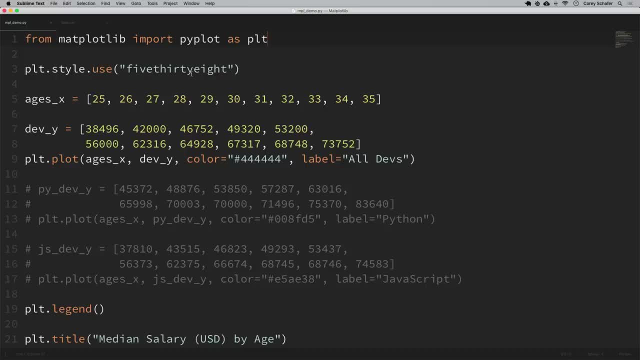 data from a CSV instead of just having our data directly within our Python script, because most likely, when you're plotting data, the data is going to be coming from another source, like a CSV file. Now I would like to mention that we do have a sponsor for this series of videos. 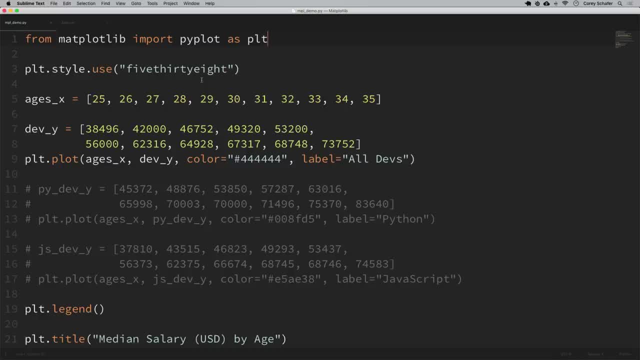 and that is Brilliantorg. So I really want to thank Brilliant for sponsoring the series, and it would be great if you all could check them out using the link in the description section below- and support the sponsors- And I'll talk more about their services in just a bit. So with that, 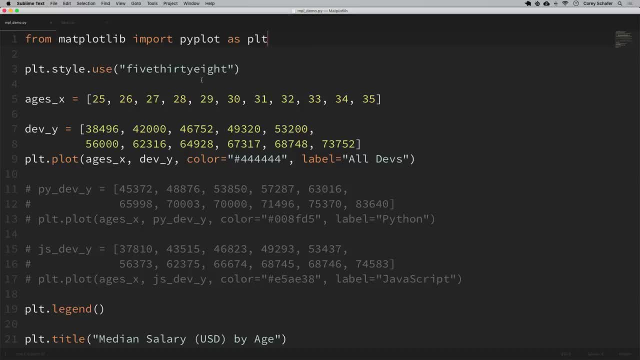 said: let's go ahead and get started. Okay, so in the last video we learned the basics of Matplotlib and how to plot some data and customize our plots in different ways. I have a stripped down version of the code that we wrote in that video opened up here in my editor and I'll have.